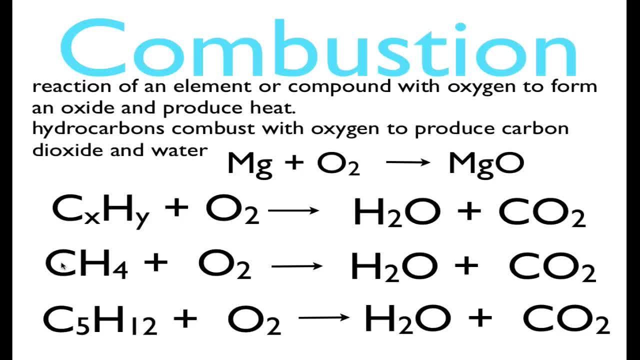 The first thing we want to do is balance the carbons, and the hydrogens and the oxygens will do last, So we're going to do the carbons first. So you can see, here we have one carbon and one carbon, so we don't need to do anything there. 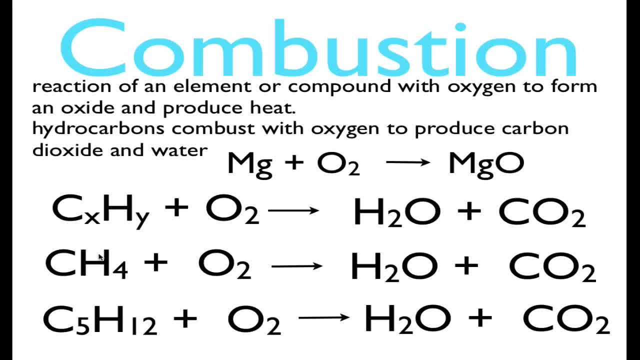 But here we have two hydrogens and here we have four hydrogens. So therefore we're going to have to add a two in front of our water so that we have four hydrogens. We put a four there, put a two there. 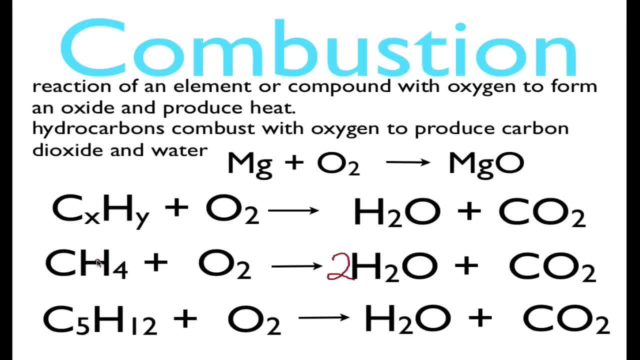 That gives us four hydrogens, Four hydrogens, Four hydrogens, one carbon, one carbon, and then we have oxygen two places over here. So we're going to add up all the oxygens So we can see two times: one is two oxygens and then we have two more oxygens over here, for a total of four. 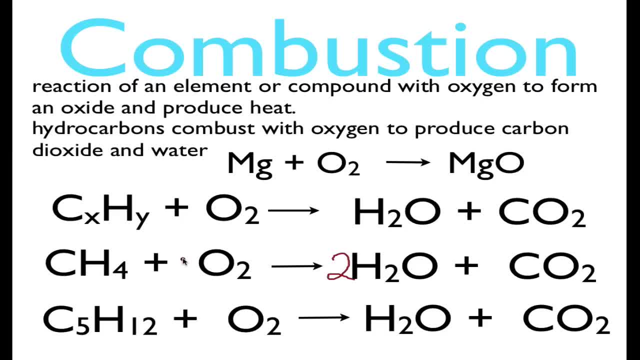 And we only have oxygen in one place over here, so we're going to have to put a two in here, so that we therefore have four oxygens. Okay, so that's the combustion reaction for methane. Now here we have C5H12.. 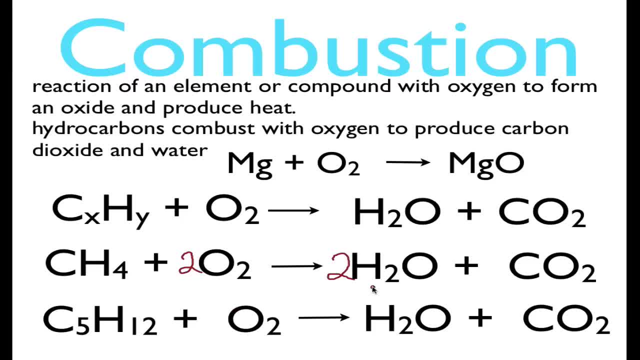 This is pentane, and we have pentane reacting with oxygen to form water And carbon dioxide again are typical products for our combustion reaction. Now let's balance this one. Here we have five carbons, so the only thing we can do is put a five over here. 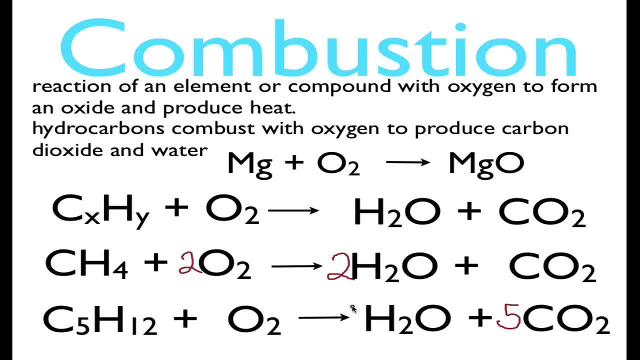 And then we have 12 hydrogens. Well, the only thing we can do is put a six right here to get 12 hydrogens. Now that means we have six oxygens and over here we have five times two is ten oxygens, for a total of 16.. 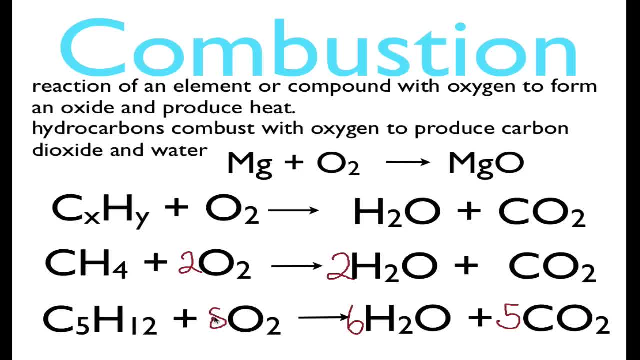 So, therefore, we're going to put an eight right there, like that, We'll give it 16.. So that is, This is the balanced chemical equation for the combustion of pentane in oxygen. Now, of course, no combustion reaction video would be complete without some demos of some combustion reactions. 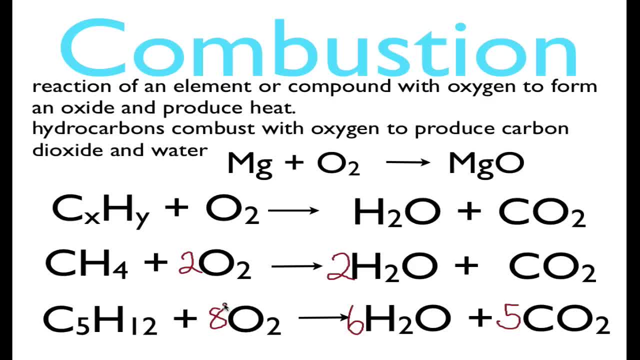 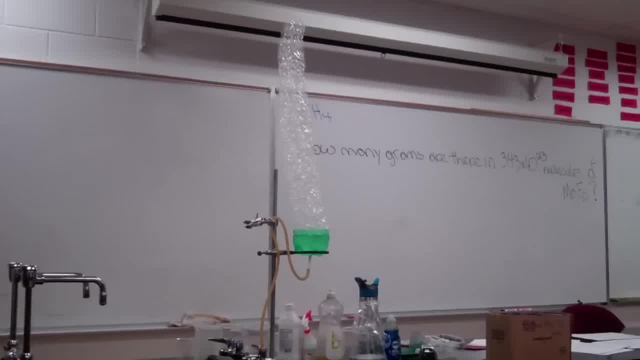 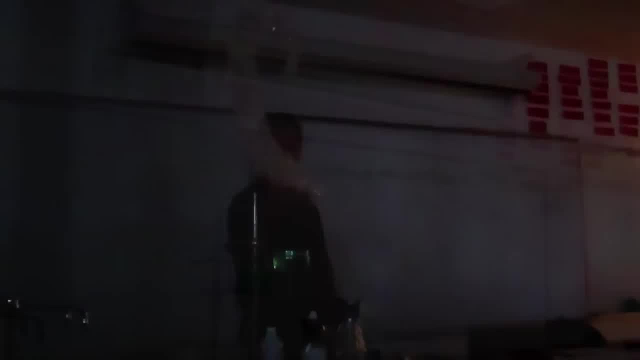 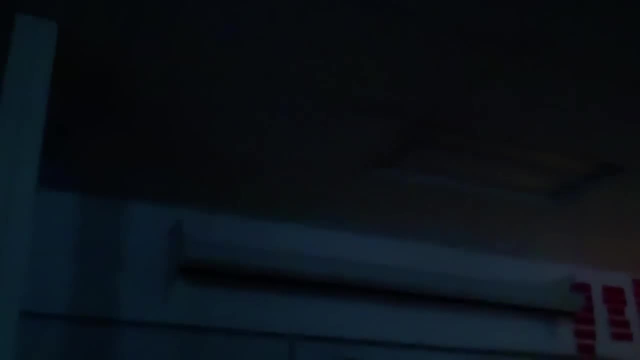 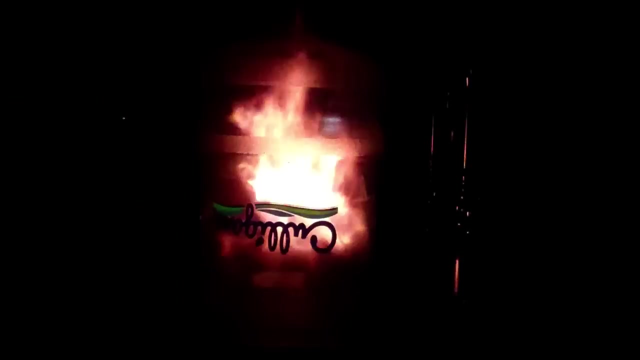 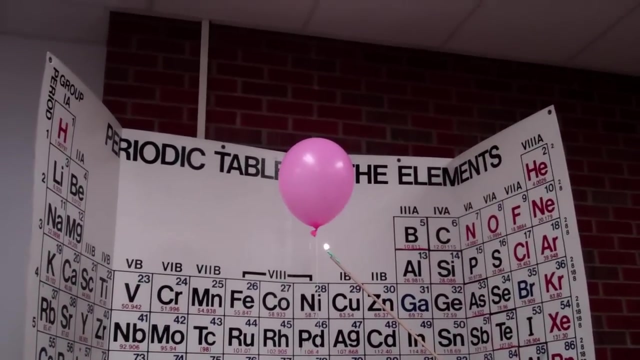 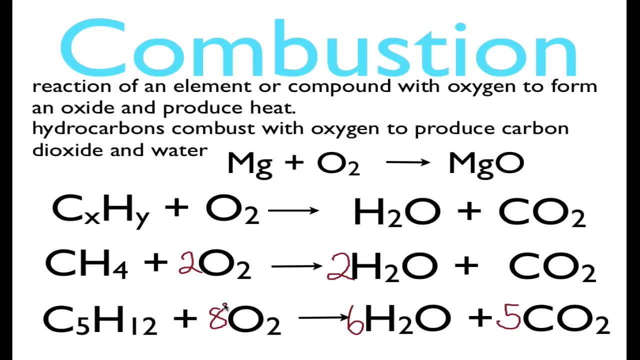 So let's go and do some and then we'll just come back and wrap things up. Okay, let's release some energy, Okay. Okay, we did all those. Those are really good. That's the methane mamba, that's the hydrogen gas in the balloon, and we did the whoosh bottle and those are all really fun reactions to do, and everybody loves to light stuff on fire. 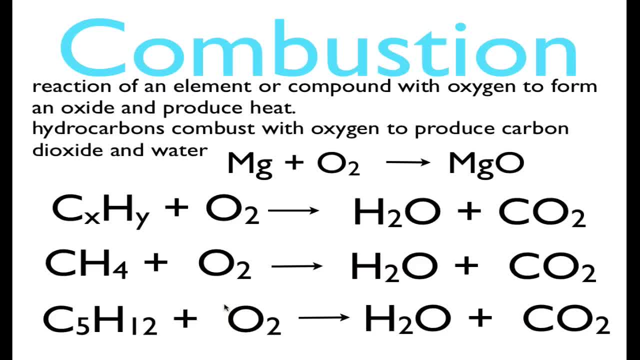 Okay, so thanks for watching, have a good day and we will see you next time. 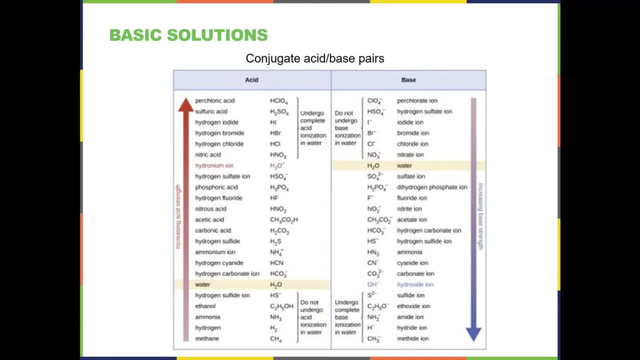 In this section we want to focus on basic solutions. So we've spent a lot of time talking about acids and Ka and Pka and things like that, But in this section we're going to talk about Kb and Pkb. So this slide is a little bit faded, so it's not the best, But we talked before about how. 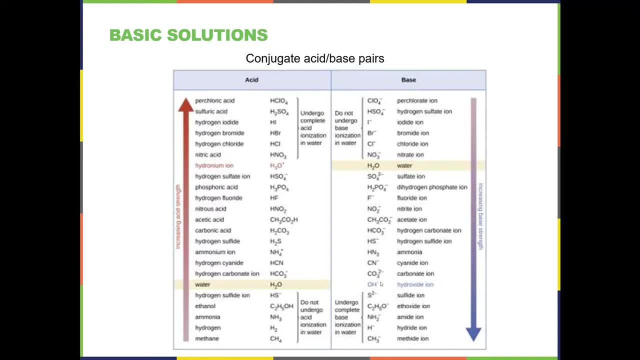 1a, metal hydroxides, lithium, sodium and potassium were strong bases And things that form hydroxide ion in solution are strong bases. But there are also many other types of bases, as you can see on this list And as we go down we are increasing them in strength. 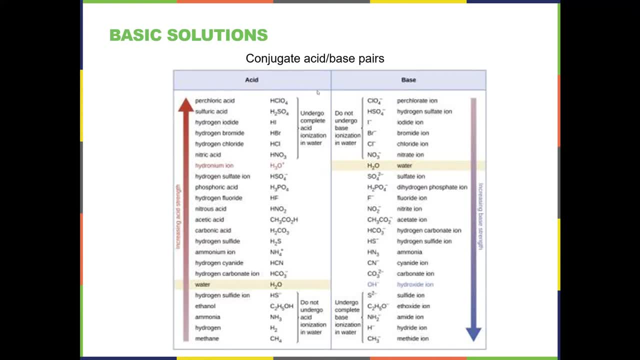 There's a couple of things to notice here If you look at the strong acids. so up here we have our strong acids And then we look at the conjugate base of those strong acids. These are all very weak bases. Said another way, the acid strength goes up, this way the base strength goes down. 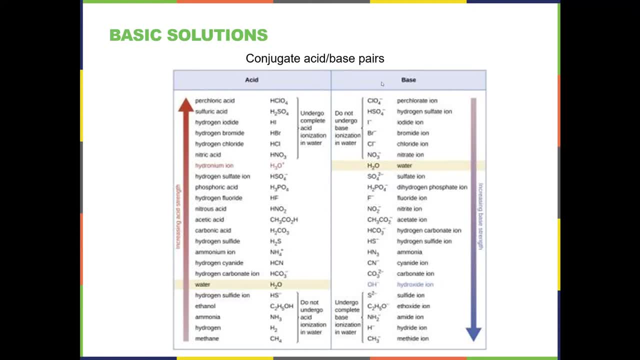 This way. So these strong acids have very weak conjugate bases, And that makes perfect sense, right? If HCl really wants to get rid of a proton, then Cl- isn't going to strongly want to take a proton, because then it would form HCl, which really wants to get rid of a proton. So this: